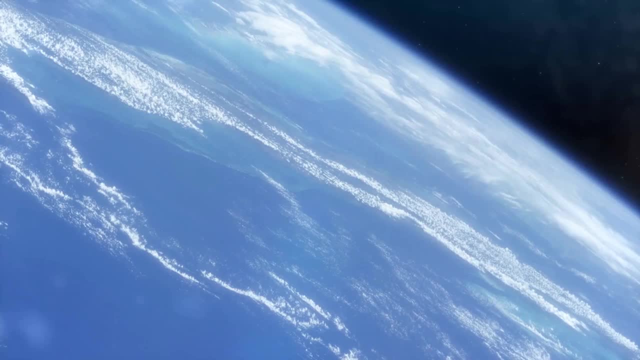 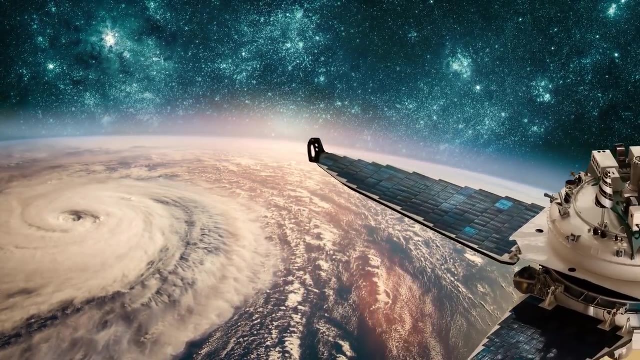 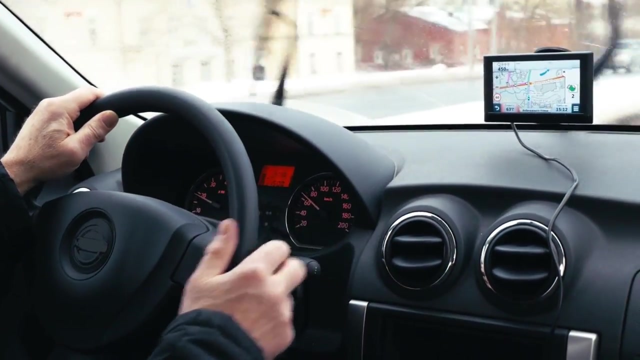 Because they were closer to the curvature of space-time due to the earth's mass, so time flowed more slowly for them. Microseconds might seem incredibly insignificant to our day-to-day lives, But they are. But understanding time dilation is crucial to making something like the GPS satellites work. 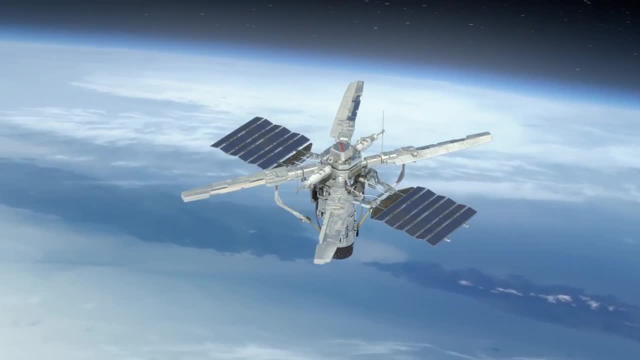 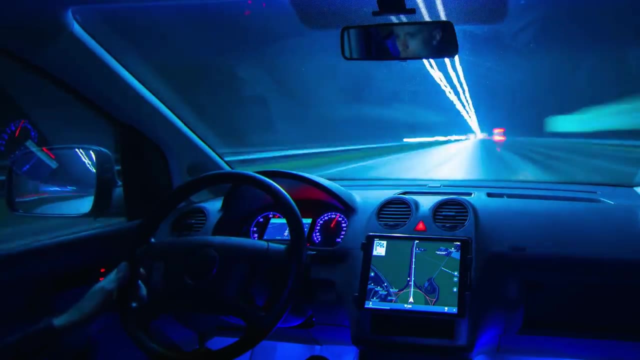 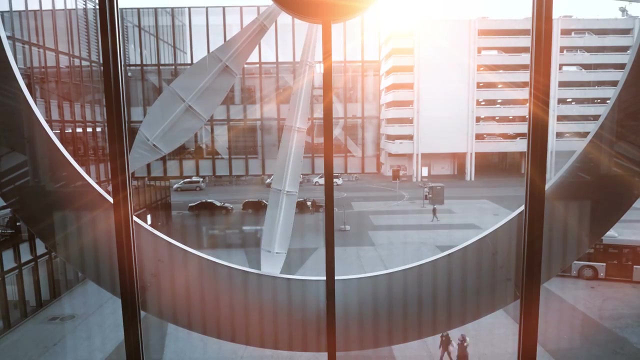 Without taking into consideration the effects of general relativity, errors in global positions would continue to accumulate at a rate of about 10 km each day, rendering GPS worthless. Considering this fluidity and somewhat counter-intuitive nature, time might seem nothing more but an illusion. 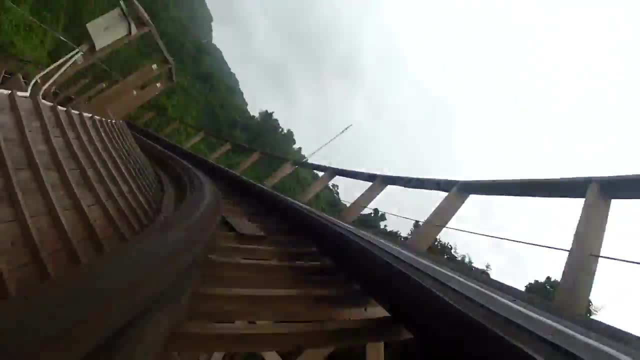 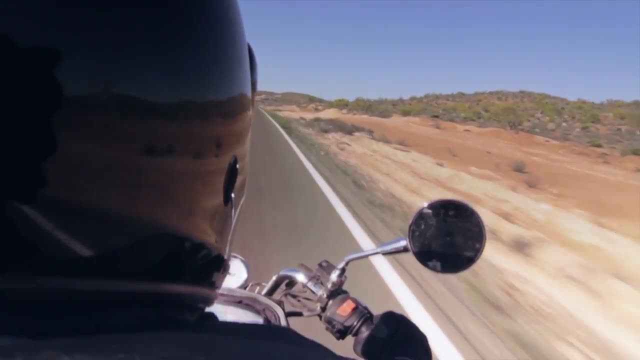 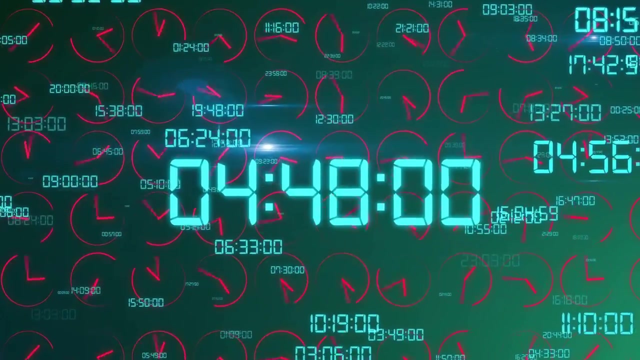 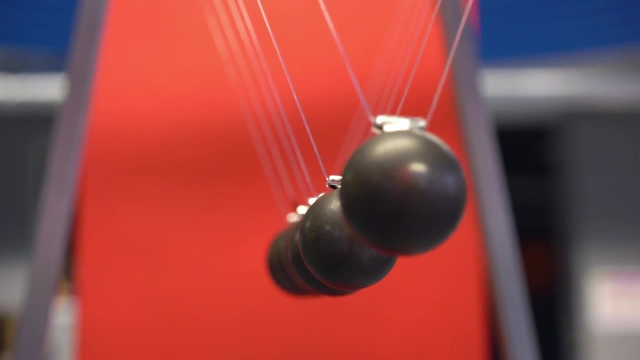 Especially because time is used to define other quantities, such as velocity, And defining time by velocity of matter, for example, seems like circularity of definition. Not only that, the operational definition does not address what the fundamental nature of time is. It doesn't entail why events can happen forward and backwards in space, while events can only happen forwards in time. 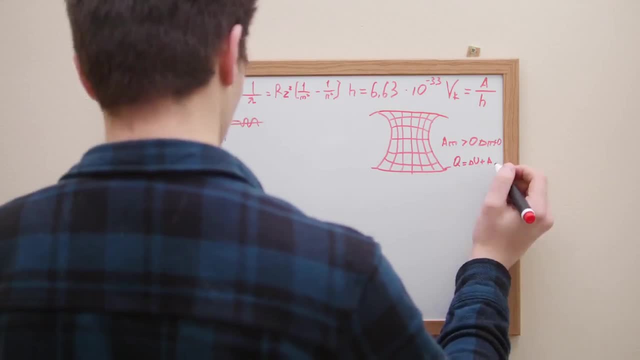 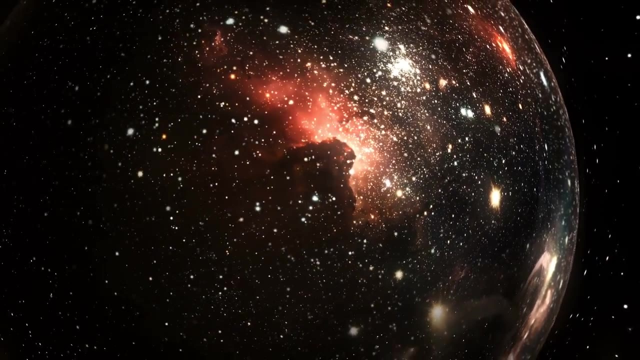 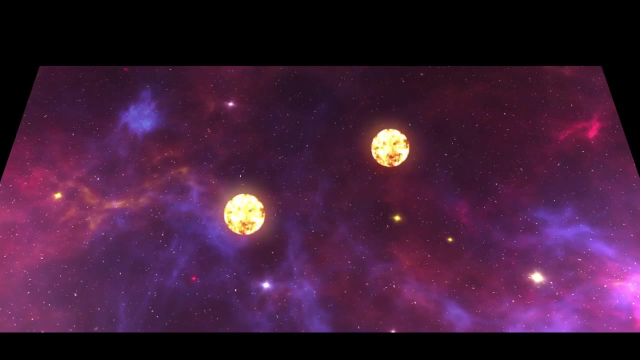 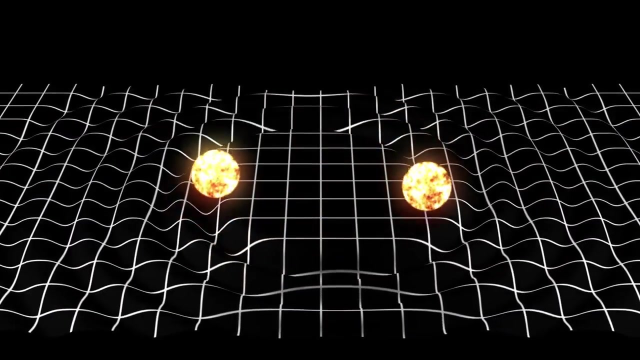 Investigations into the relationship between space and time led physicists to define the space-time continuum. General relativity is the primary framework for understanding how space-time works. Through advances in both theoretical and experimental investigations of space-time, it has been shown that time can be distorted, particularly at the edges of black holes. 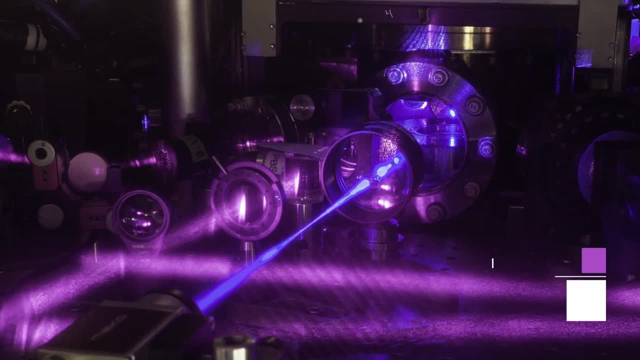 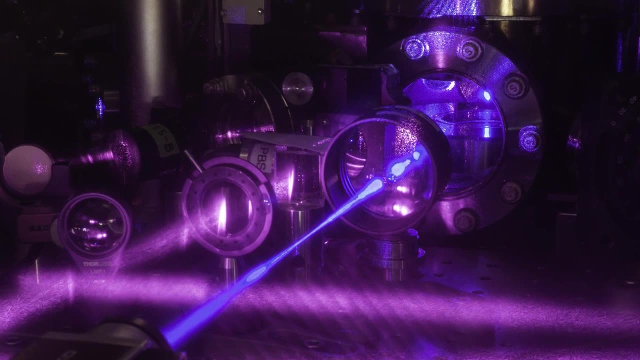 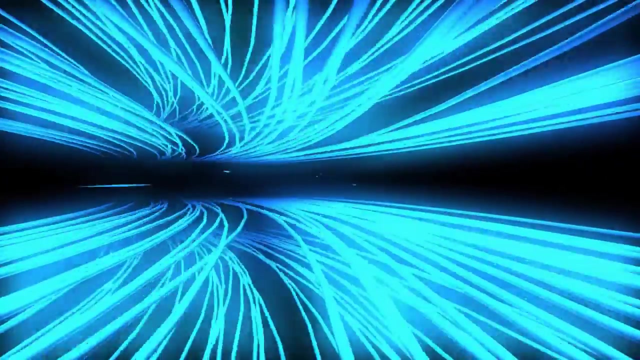 The story of time can be distorted, particularly at the edges of black holes. The Strontium atomic clock is the most precise clock ever devised by humans. It's accurate to within a second, over 15 billion years. Yet, because of Einstein, we know space and time are fluid and are affected by gravity and velocity. 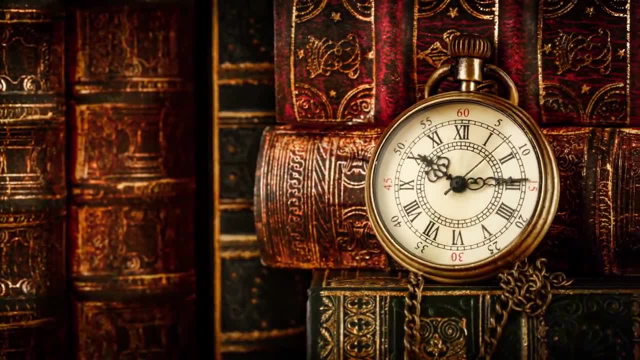 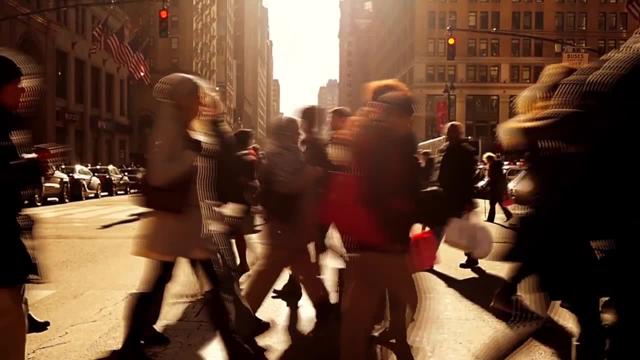 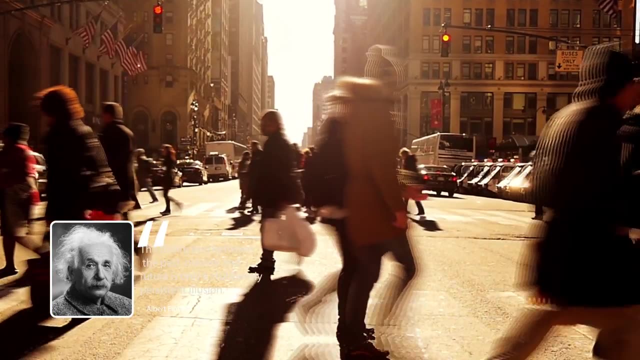 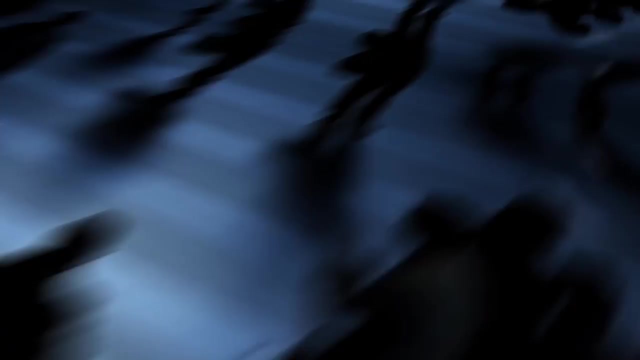 And it may make us feel uncomfortable to think. something so fundamental to our existence can be considered an illusion, But, quoting Einstein, the distinction between the past, present and future is only a stubbornly persistent illusion. Thanks for watching. Did you like this video?